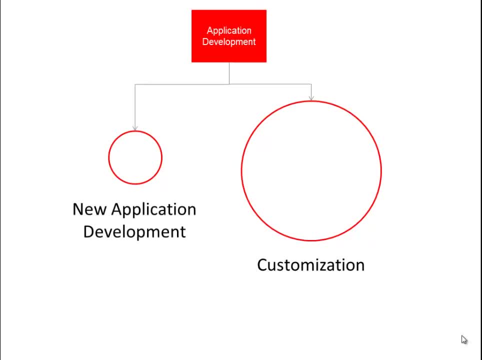 as it is a more intuitive starting point to help us understand how software is developed. Let's look at who is involved in developing new software. At minimum, we need a customer and a software developer. A customer is generally a person or group, or a company. 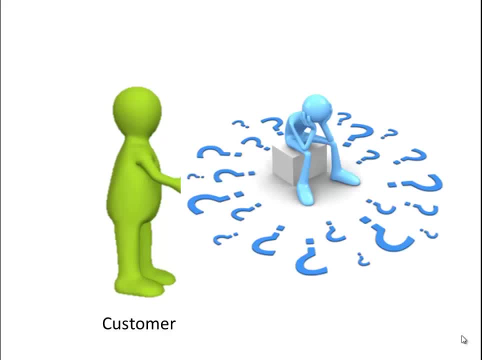 who has a problem and believes that software can somehow help some or all of that problem and is willing to invest money to develop new software. A customer wants software because it helps them do something faster, cheaper or better. Then there is the software developer or programmer. 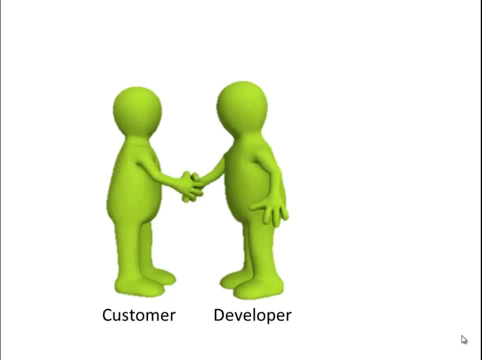 who has the programming skills and time to build software needed by the customer. Typically there is a team of programmers And, of course, many other roles like a project manager, business analyst, testers, But for now let's keep it simple and talk about only these two types of people. 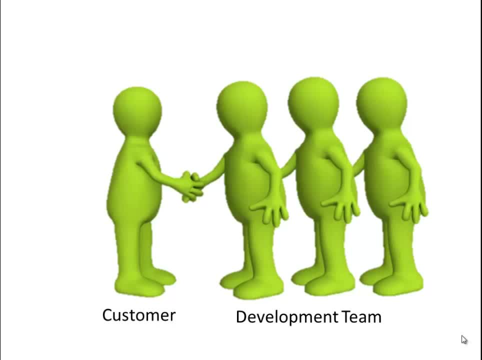 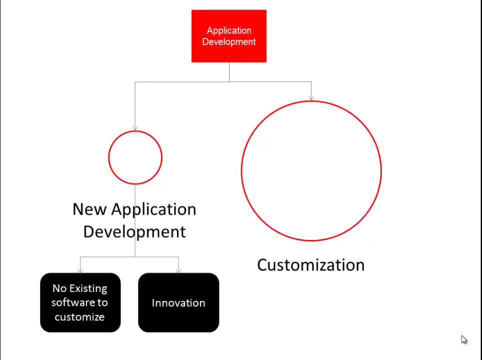 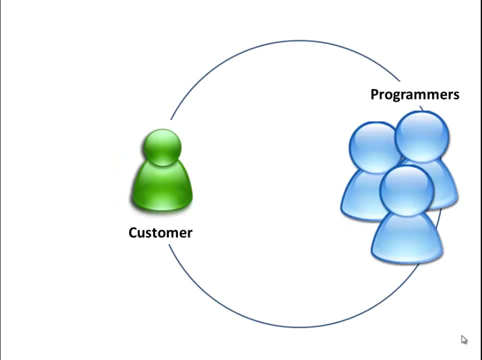 New software is developed when there is no existing software that meets some or all of the customer's requirements, Or the customer wishes to invest in innovation to create something new. Let's look at how software gets built. In the most simple case, software gets built like this: 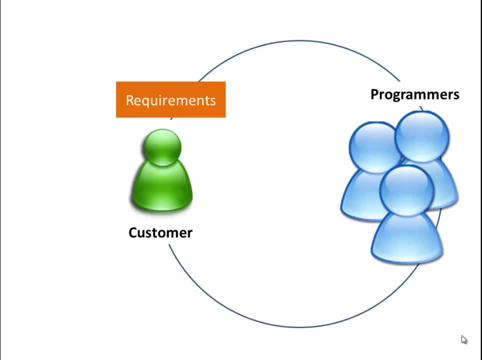 A customer explains his or her requirements to the development team, who then design and develop the software. The software, once completed, is made available to the customer, who then tests it and finally deploys the application so that others can begin to use the software. 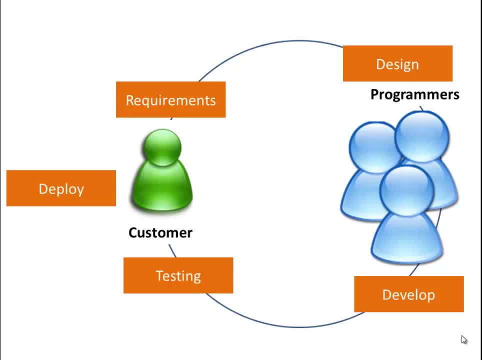 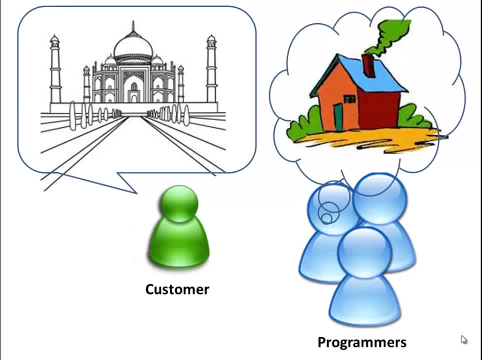 But here's where things start to get interesting. Let's look at what happens if the customer didn't explain the requirements well, or the developer didn't fully understand the requirements. Quite understandably. if the requirements were not accurate, what gets designed and developed and tested will also not be correct. 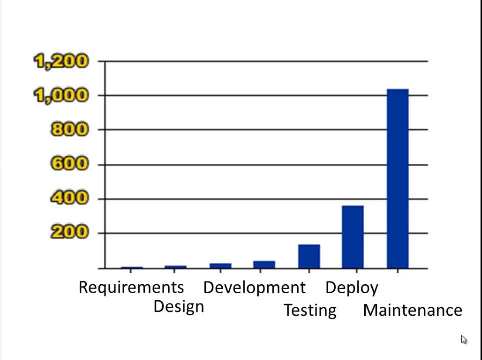 Here's a chart which shows the cost of fixing requirements errors in a project. As you can see, it's relatively easy to fix requirements errors early in the project and a lot more expensive to fix it later in the project. But how big an issue is this? 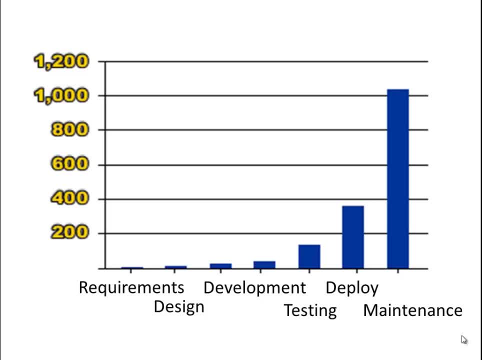 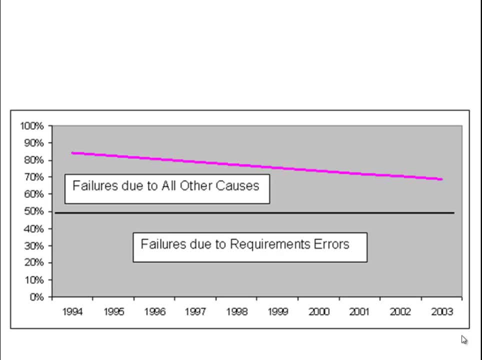 How many projects globally are affected by not getting the correct requirements? Studies have shown that about 70% of all software projects fail to get delivered on time, within budget or to the quality that the customer expected. Let's pause here for a bit and think about what this means. 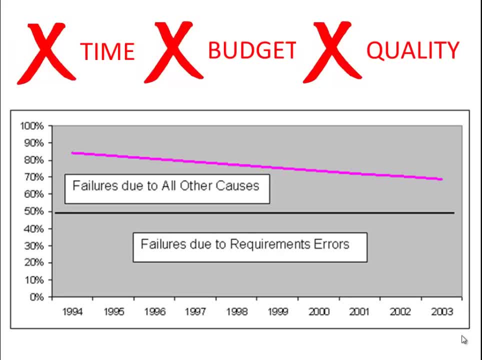 If you are currently involved in a software project, it means that there is a 70% chance that your project will be late or over budget or not be delivered to the quality that's expected, If we think in terms of the amount of money spent each year. 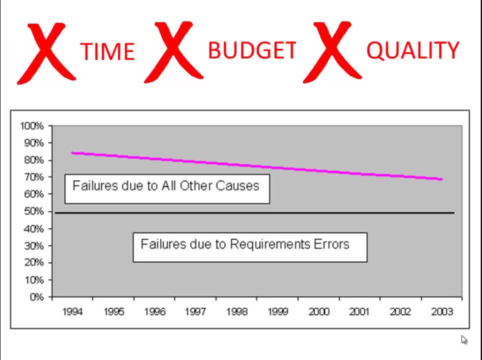 on all software development across the world, that adds up to several millions, sometimes billions, spent on failure. We rarely see such low success rates in any other engineering discipline. So what's going on here? Why is software development not like other engineering disciplines? 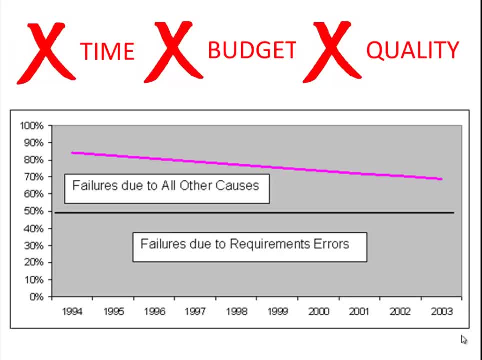 Compared to other engineering disciplines like mechanical or civil engineering, which have been around for hundreds of years, computer and software engineering is relatively new, only at 50 years. Nevertheless, we would assume that somehow we would have figured out how to improve our success rates in the past 50 years. 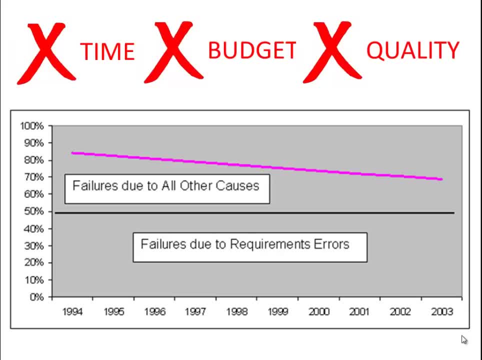 If you look at the failure rate from 1994 to 2003,, we appear to be improving, But it doesn't seem like we have gotten past the 30% success rate and 70% of projects still appear to be in trouble. 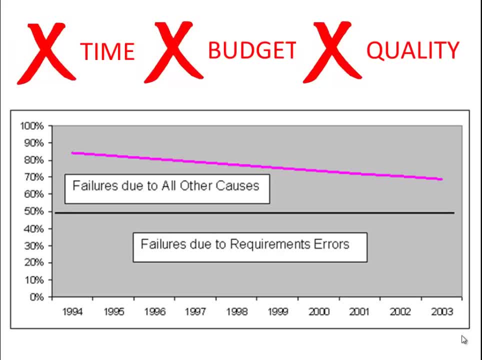 Seems a bit depressing, but is this really true? Are 70% of projects in fact late or over budget, Or is this just a perception? We will discuss the answer to this question in more detail in a separate video, But for now, 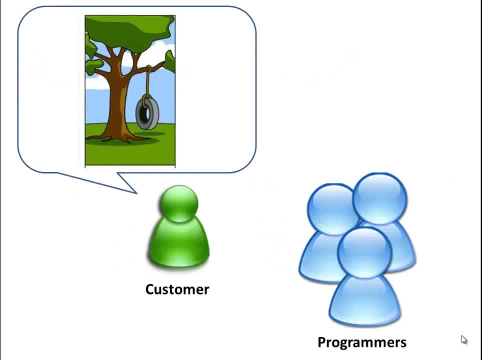 let's focus on the first and the most important step in building software on time and on budget and to a high quality: Getting the customer's requirements right. Please join me in the next video as we look at different ways to understand the customer's requirements. 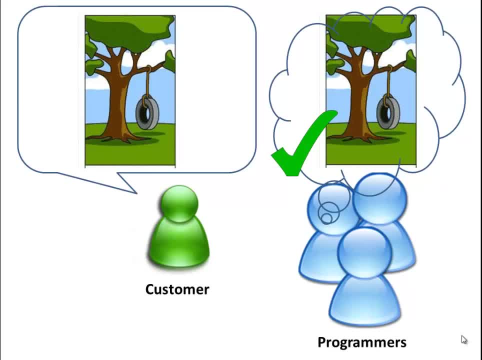 and look at ways to increase the success rate of software development projects.